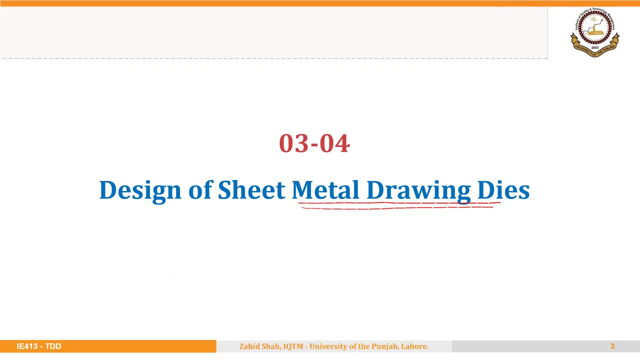 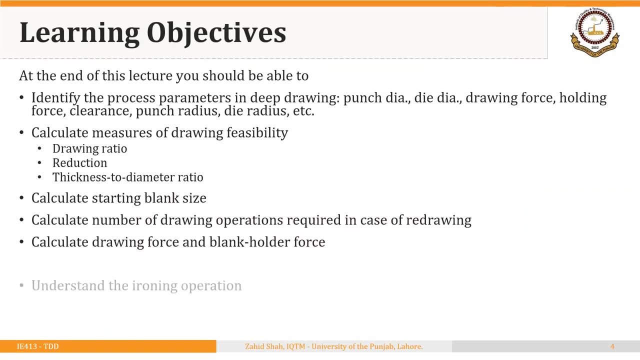 as well as processing and analysis of sheet metal drawing, and that is also called deep drawing. So at the end of this lecture you should be able to identify the process parameters in deep drawing. So they include punch, dia, die dia, drawing force, a blank holding. 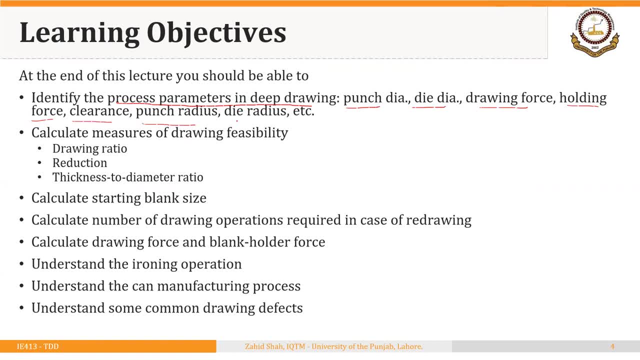 force clearance between punch and die, punch radius, die radius, etc. We should be able to calculate measures of drawing feasibility. They include drawing ratio reduction and thickness to diameter ratio, And you should be able to calculate starting blank size. So, just like bending operations, we need to 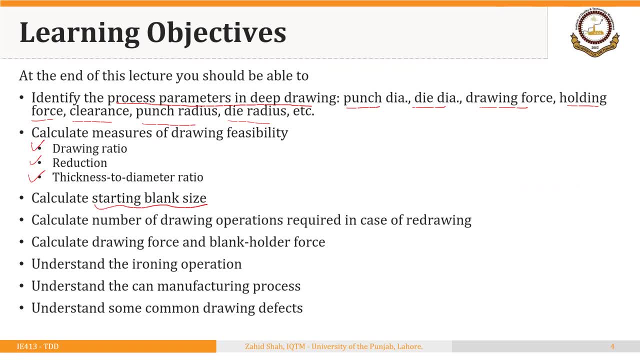 calculate accurate size of the blank before the drawing operation is to be performed. You should be able to calculate number of drawing operations required in the case of redrawing or wear �도qu. También hay que ser utilizados más de una operación de dibujo. 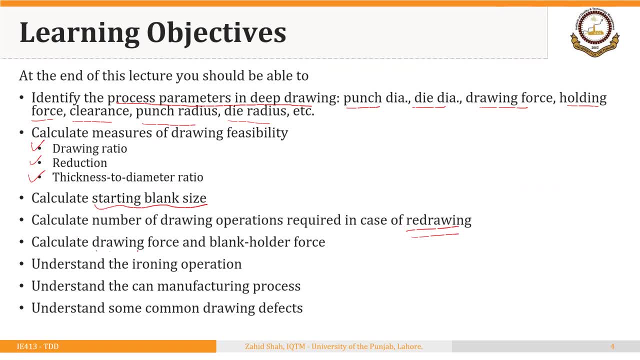 You should be able to calculate drawing force, force that is required to perform drawing operation, along with blank holder force. Then we will discuss the ironing operation, Another process required. It can be performed after a deep drawing operation. Then we discuss the process to making a can using a drawing tool. 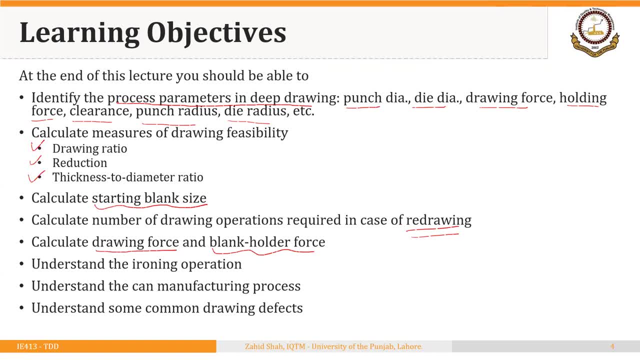 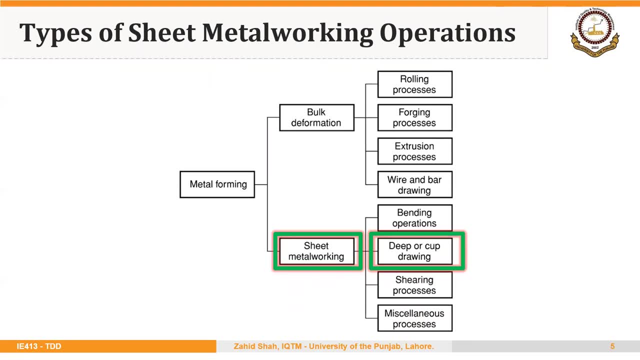 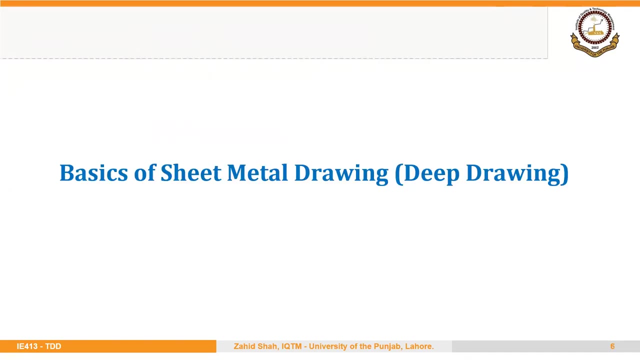 an application of deep drawing process. and finally, you should be able to understand some common drawing defects. So we are discussing sheet metal working processes. we have discussed shearing or cutting processes, we have discussed bending processes and now we are focusing on deep or cup drawing. So first we will discuss some basics of sheet metal drawing. that is also called 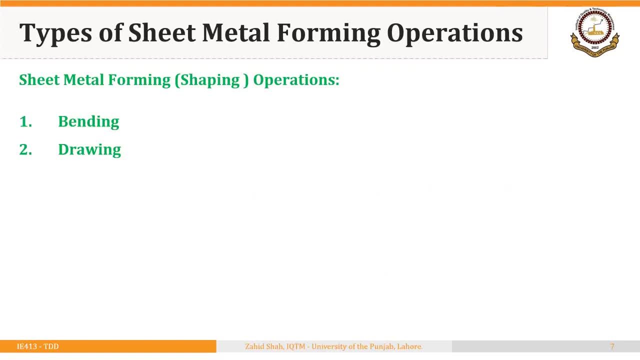 deep drawing. So this is one of the shaping or forming processes in sheet metal working. So we have discussed one example of forming processes in sheet metal working. they are the bending processes and now we are going to focus on the drawing processes. So deep drawing is sheet metal. 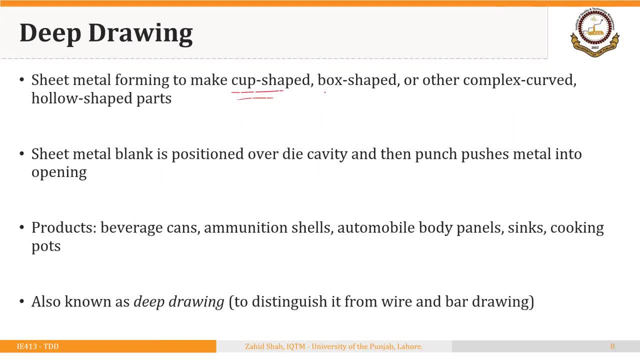 forming to make cup shaped or box shaped or other complex curved, hollow shaped products. As you will notice that these products are mostly either shallow products or deep products, but they are hollow from inside. Sheet metal blank is positioned over the die cavity and then punch pushes metal into the die opening. So the blanking is actually the primary process. 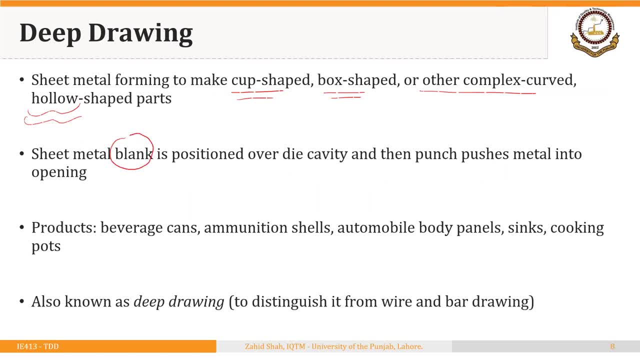 for sheet metal drawing or deep drawing. The process of deep drawing include beverage cans- that is the classical example of deep drawn product- ammunition shells, automobile body panels, sinks, cooking pots, etc. This process is called sheet metal drawing or deep drawing, especially to distinguish it from. 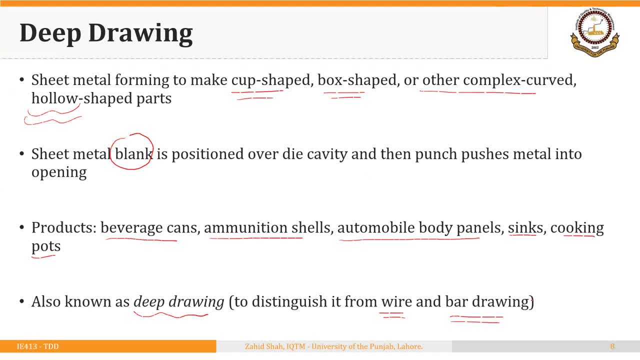 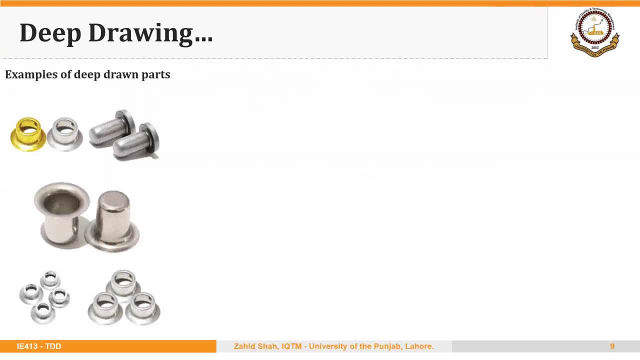 wire and bar drawing and they are also the example of deformation processes. but although they have the same name, the drawing operations, but they are very different from sheet metal drawing or deep drawing. There are some examples of deep drawn parts. you could see that this part is drawn up to certain. 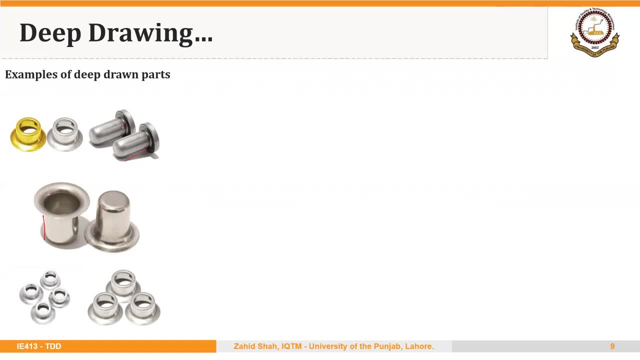 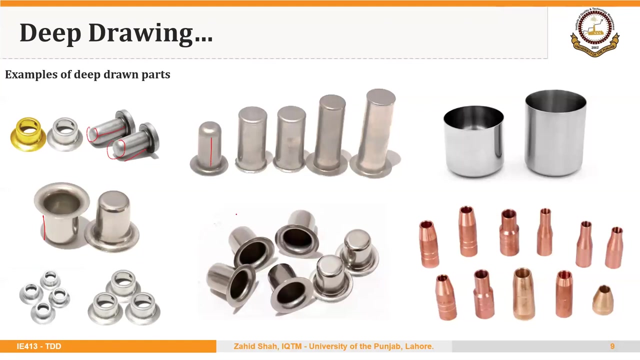 depth. same is true about this part as well as this one. some of them are hollow from both sides, I mean they don't have bottom, but some of them do have a base or bottom. So you could see that in all cases the part is drawn. so this is the drawn portion of the part. so this is the portion of the blank that is drawn into the die. 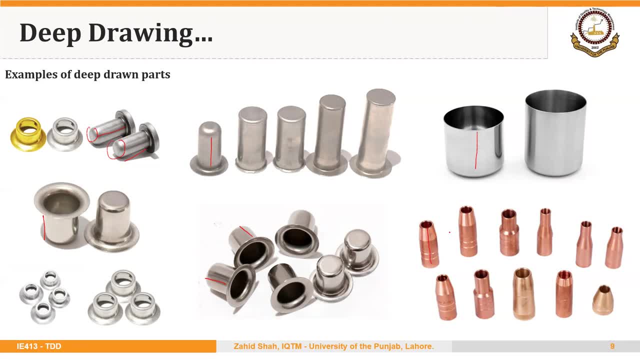 So a couple of things that you might notice in all these parts. one is, of course, they are hollow from inside, and the second thing in the deep drawing process is that the surface is hollow. thing in the part shown on the slide is that they are symmetric. so these parts are symmetric about. 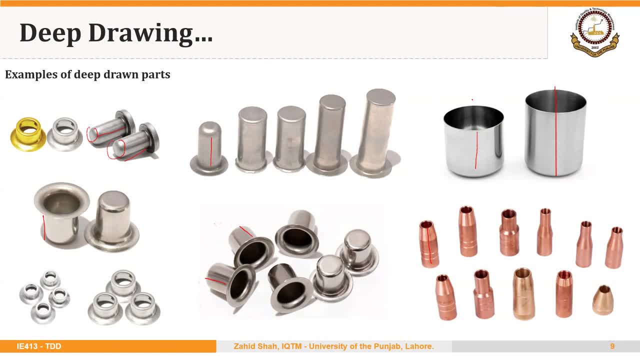 certain axis, so this part is symmetric about this axis. this part is symmetric about certain axis like this: this part is also symmetric, so these parts are symmetric about certain vertical axis, but that is not necessarily in all cases. but these are the simplest examples, the simplest parts that we can make using deep drawing, and in this case, all these are symmetric. 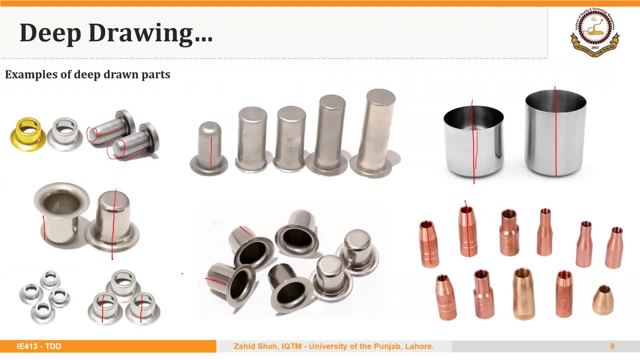 about certain vertical axes, but of course we can make more complex parts than these. in this series of lectures on deep drawing, we will primarily focus on simple shapes like these. so we will be having a flat blank that will be drawn into simple shapes like these, the shapes that have a certain height and certain diameter, or at some 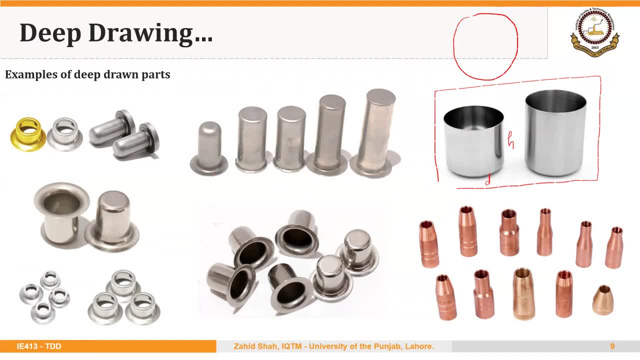 time we might be looking for slightly more complex shape like this one that, apart from a height, also has a flange or a collar. so once you are able to understand the drawing process for these simple shapes, it is easy to extend the concepts to more complex shapes. 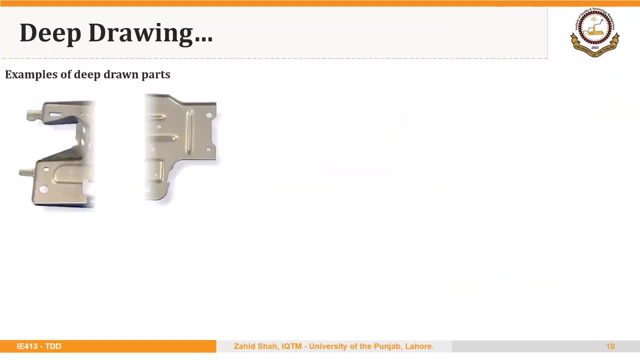 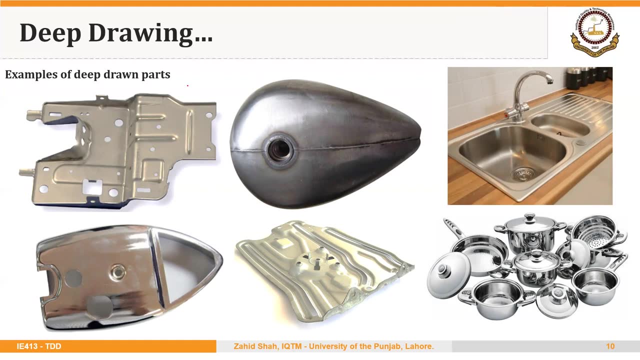 and of course we can make more complex shapes like the ones shown on this slide, so you could have certain parts of the cars and automobiles. the iron, the fuel tank of the motorcycle or, similarly, the fuel tank of of car can be made using deep drying process, the sinks or cell utensils. so these are just few of many. 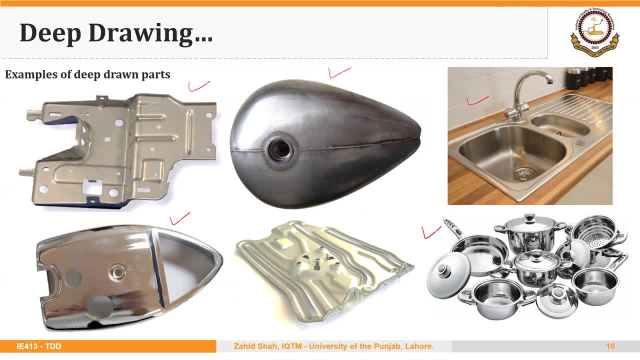 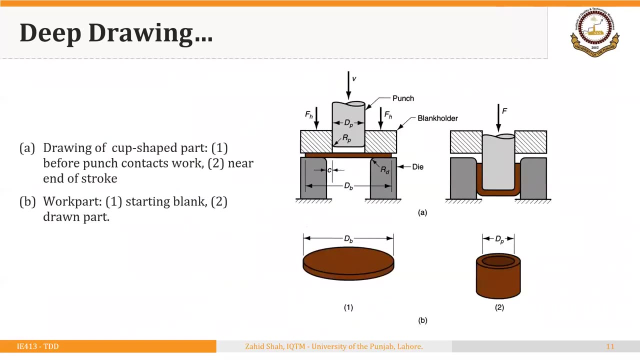 examples of the parts that can be made using deep drawn using deep drawing process, and these parts mentioned on this slide are relatively more complex than the ones on the previous slide, so this figure will help us to understand some important process parameter in deep drawing process for a simple shape like this. as i mentioned that we will primarily focus on this. 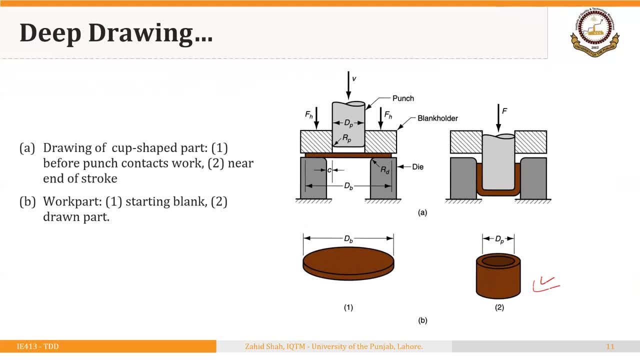 simple shape, a plane shell that is drawn using a starting flat circular blank. this shell will have a certain diameter and certain height, so important process parameters are the diameter of the punch, so that will determine the inner diameter of the shell, and then there is of course a certain diameter of the die. 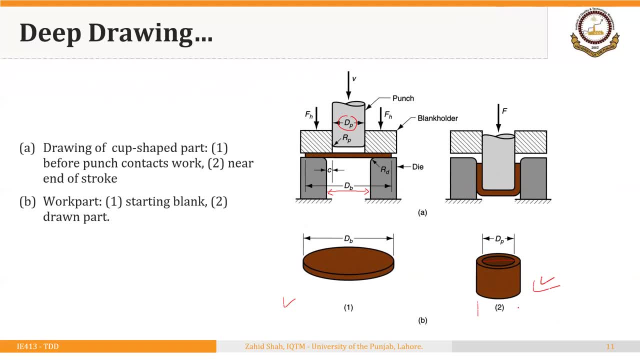 that will determine the outer diameter of this shell. this diameter, then we are having a certain radius at the bottom of the punch. this radius, there is actually needed to be a certain radius in order to avoid tearing of the blank, and similarly, we need to have a certain radius for the die as well. so these two radii are important. 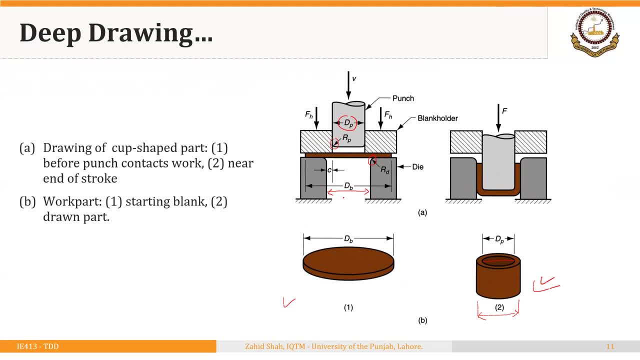 so so far we have seen two dies: the diameter of the punch, the diameter of the die, the radius on the punch and radius on the die. so this radius on the punch will determine the inner radius of the shell and this radius on the die will determine the outer radius at the bottom of the shell. then, of course, just like bending, we need 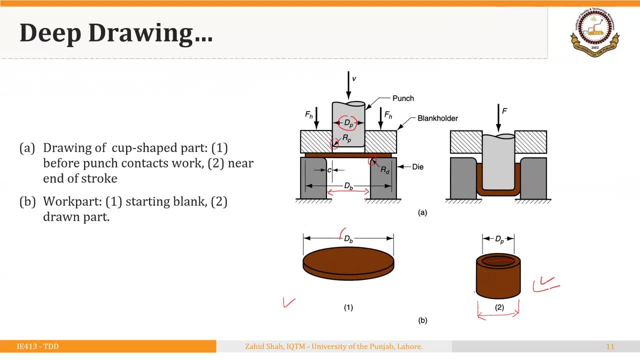 to have a certain um diameter of the blank and it needs to be accurately calculated. so that was the most important task required to determine what the size of the punch should be, and the last task that we have to do is to determine how the size of the punch should be. 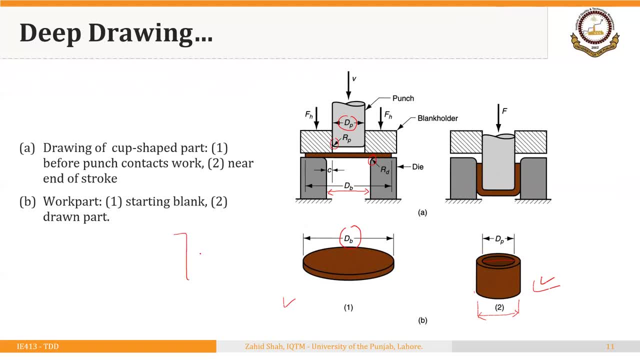 and we have to determine what the size of the punch should be and what the dead size will be. so this was the one of the infamous aberration of the punch in the digital or digital art of the caldera. you see the PERFORMANCE function here that has to do with the cutting on the punch. in the digital art of the punch. 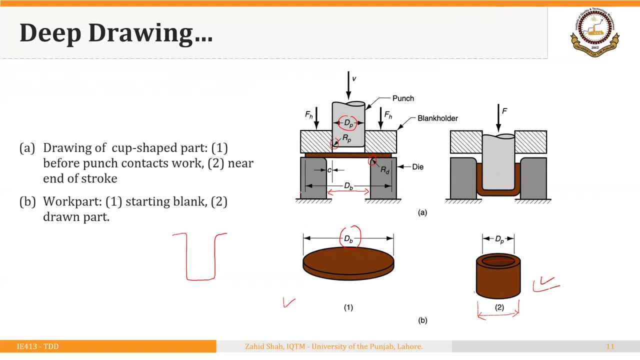 so the potential value of the punch. when you cut a punch it will be 9, 2, 3, 4 and so on, and if you plot the die in this way then you will see that the pattern is drawn into the die. you get the required shape for the parts that have some caller or flange. generally the scantry operation is performed- that is called the trimming operation- to get the desired size of these flanges or collar for the parts that have some collar or flange. 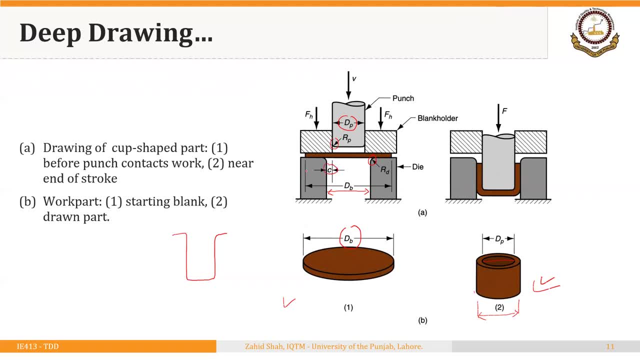 die is also very critical and it needs to be accurately calculated. For simple operations like the ones to make shapes like this cup or shell, this clearance is slightly greater than the thickness of the starting blank. An important consideration in sheet metal drying operations is this blank holder force We need. 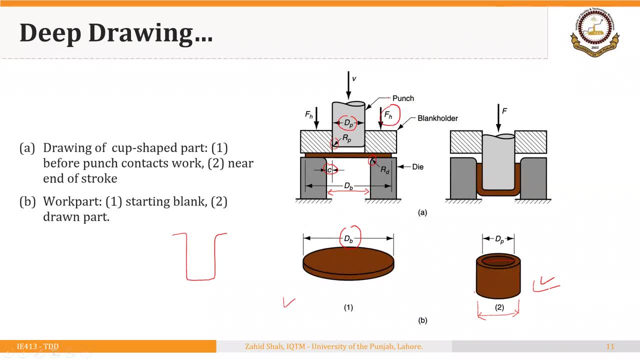 to hold the blank in position before the drying operation starts. So first this blank holder and then the drawing punch actually descends and pushes the blank into the die, actually controls the flow of the blank into the die. so this flow is controlled by this blank. 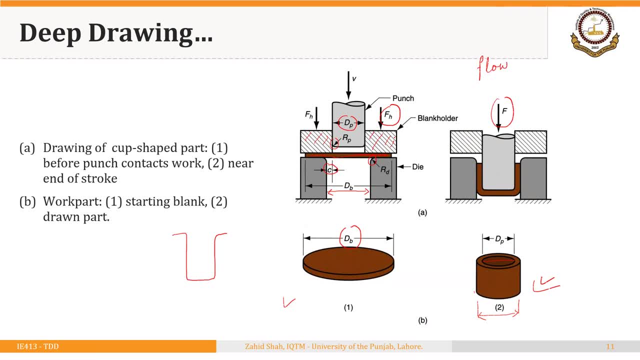 holder. so this blank holding force should not be too high so that tearing may occur, and it should not be too low so that the blank drops into the die. so this needs to have an optimum value, and this value of the blank holder force is, of course, smaller than the force that is used for. 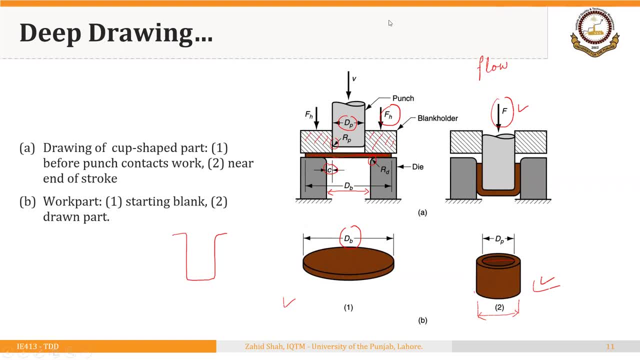 the drawing operation. so we will focus on these process parameters as we will move on. we will see how we can calculate the diameter of the starting blank, what should be the value of the radius on the punch as well as radius on the die, and we will see that, how we can calculate the this drawing. 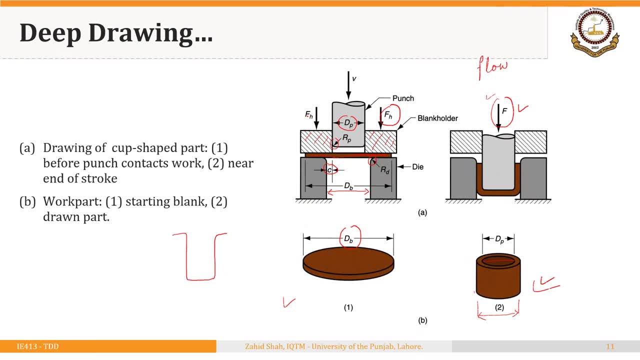 force, and then we will see how we can calculate the value of the radius on the die. and we will see, as well as the blank holder force, all these parameters: the starting blank diameter, the radius of the punch, radius of the die, the clearance between punch and die, blank holder force and 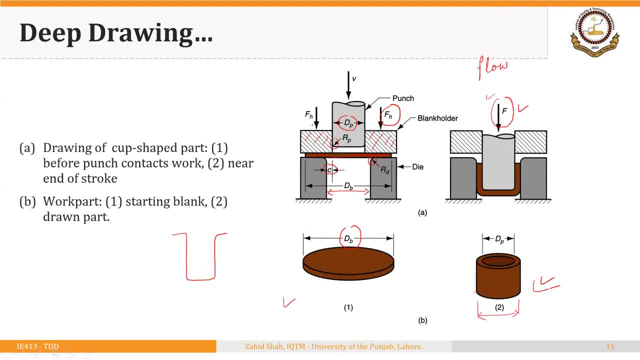 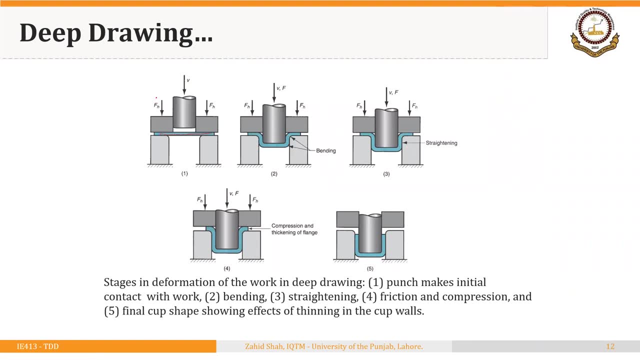 drawing force will be discussed in detail as we move on. so we have the starting blank like this that is placed onto the die: first the blank holder holds the blank into position, after that the point descends and pushes the blank into position, and then the blank holder holds the blank into position. 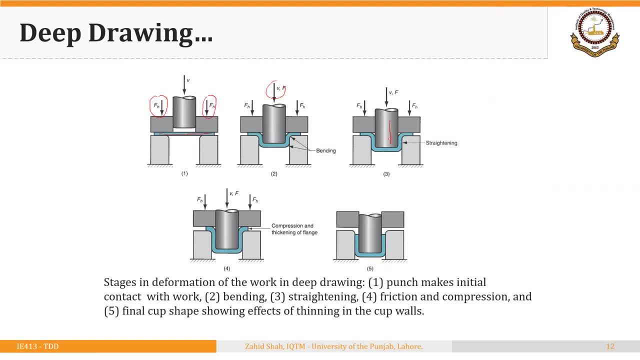 and then the blank into position one in the bank, and then this is the graph of the control. then it moves the bank into the die and as the pump pushes the blank into the die, this blank holder actually controls the slope of the blank into the die and it keeps on holding the blank.